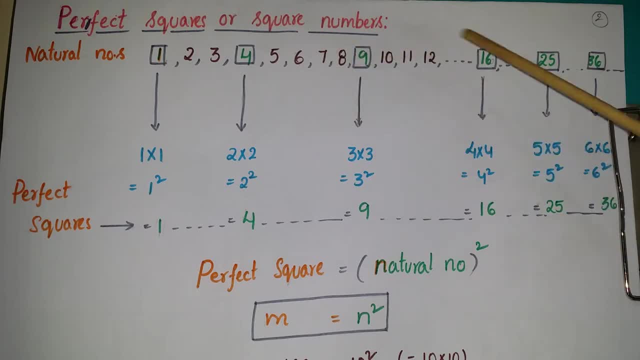 So these numbers are called 1,, 4,, 9,, 16,, 25,, 36,. these numbers are called perfect squares or square numbers. So these perfect squares we can write as 1 square, see here 2 square, 3 square, 4 square, 5 square, etc. 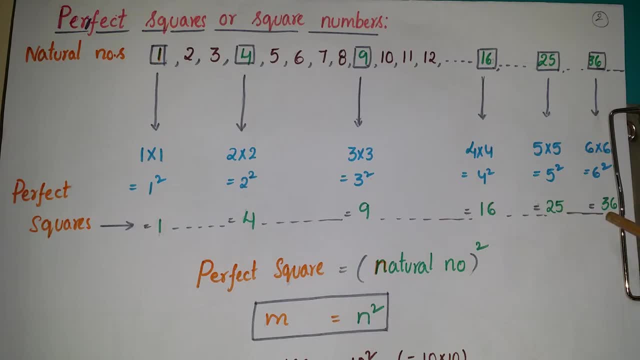 So here 1,, 4,, 9,, 16,, 25,, 36 are called perfect squares. So perfect square is a number which we can write as a square of a natural number. So perfect square is equal to natural number whole. 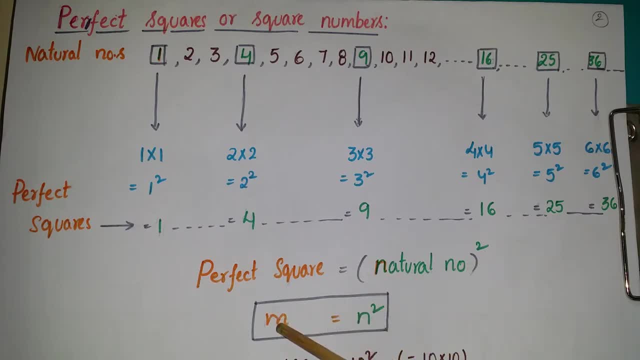 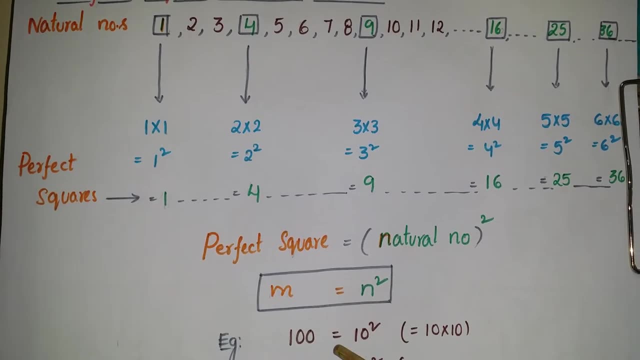 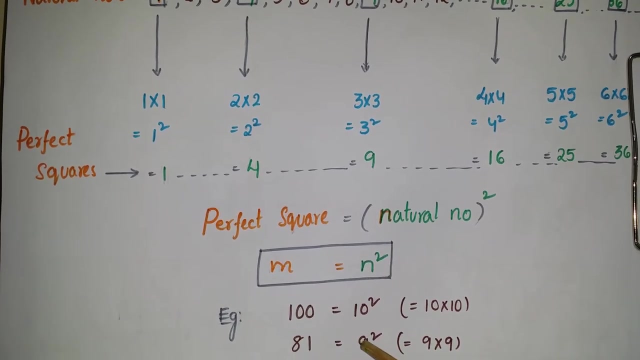 square. if we say perfect square as m, then m is equal to n square. see these examples. suppose 100: if you take 100, we can write as 10 into 10, so that is 10 square. so 100 is a perfect square. 81 also we can write as 9 into 9, so 81 is also a perfect square. 9 square. 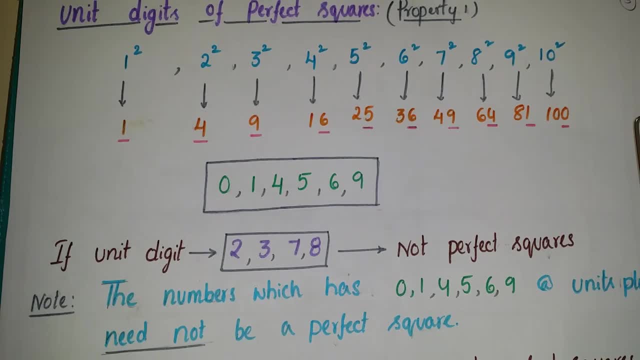 perfect squares have some properties. this is the first property. unit is itself perfect squares. see the perfect squares here: 1 square, 2 square, 3 square, 4 square, 5 square, etc. we can write these numbers like this: 1, 4, 9, 16, 25, 36, like this. if you observe these perfect squares, the unit digits are: 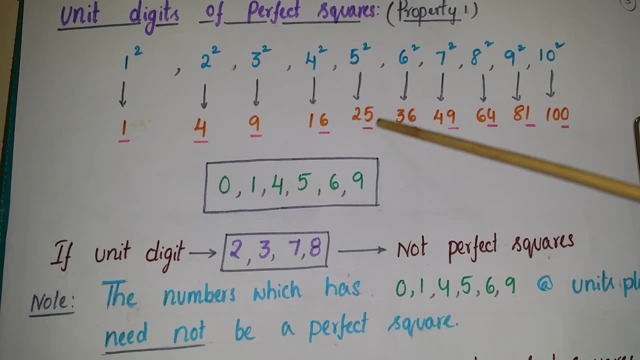 1, 4, 9, here 6, 5, 6, 9, 4, 1 and 0. so all the perfect squares have the unit digits of 0, 1, 4, 5, 6, 9. so if the unit digits are 2, 3, 7 and 8, those are not perfect squares. see the note here the numbers which has 0, 1, 4, 5, 6, 9. 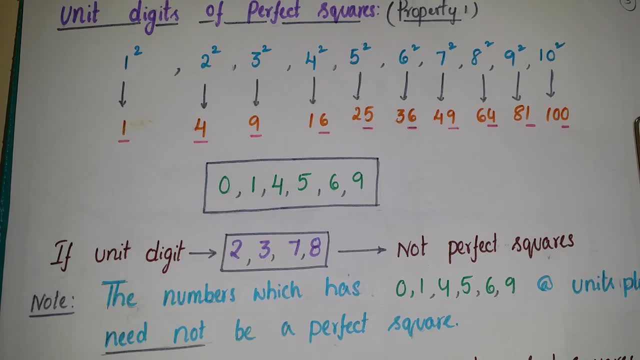 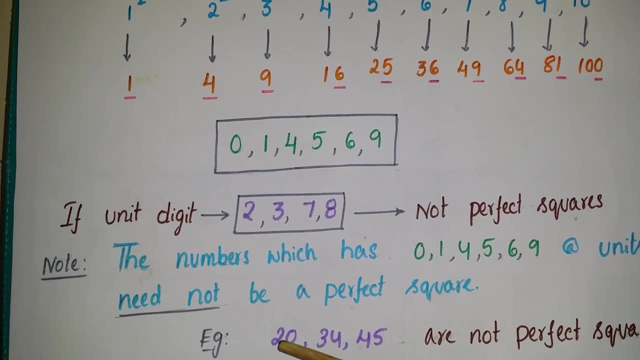 at unit place need not be a perfect square, because if you see this example- 20, 34 and 45- these are not perfect squares, but the unit digits are 0, 4 and 5.